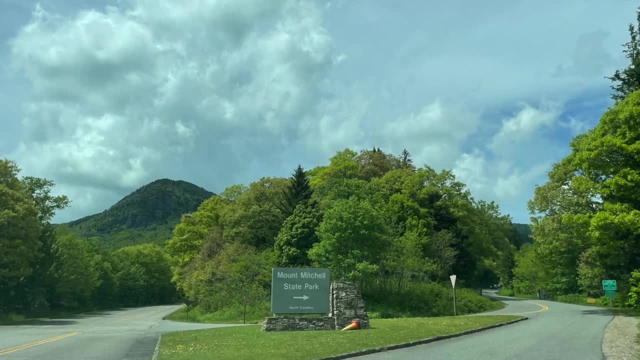 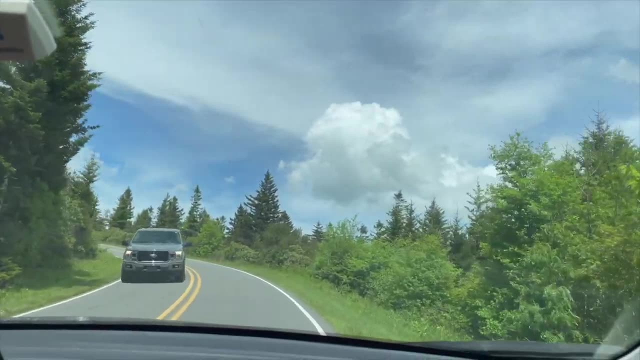 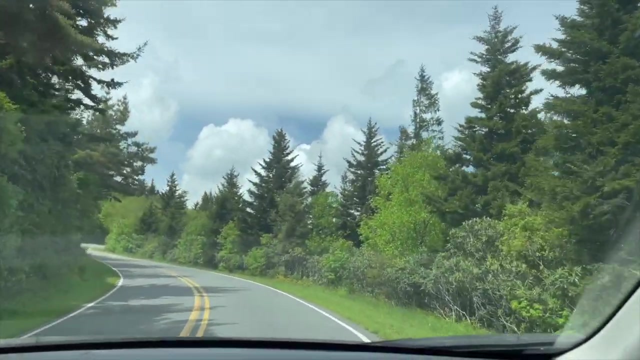 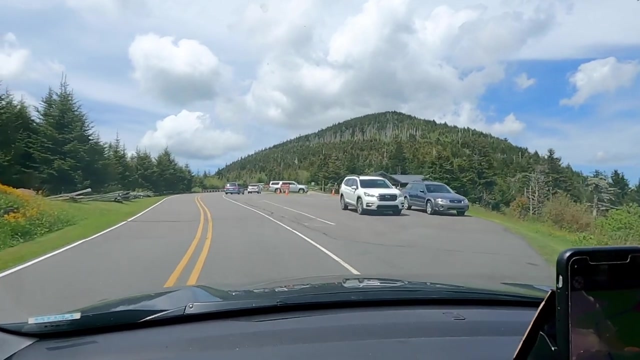 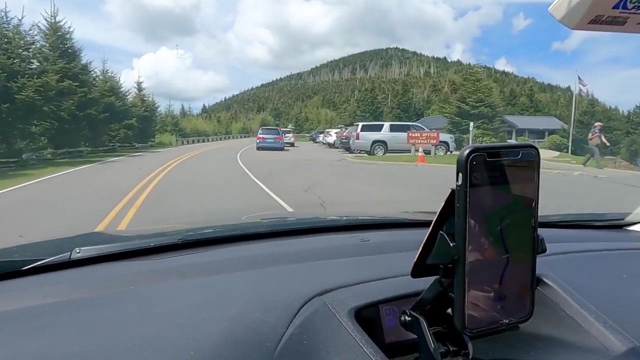 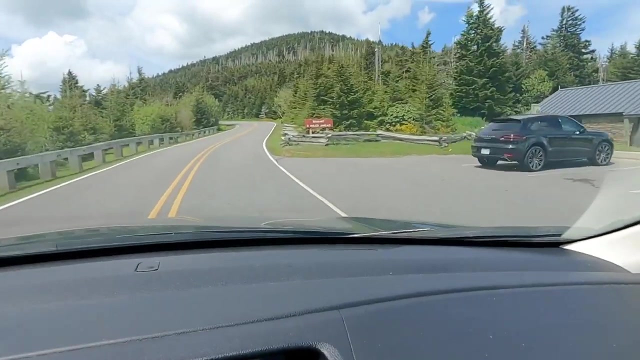 This is NC 128 at milepost 355.4. that will take us from the Blue Ridge Parkway to the summit. The The Mount Mitchell restaurant is located here, but is currently closed for renovation and will reopen in 2022.. There are hiking trails, picnic spots and a Natural History Museum. 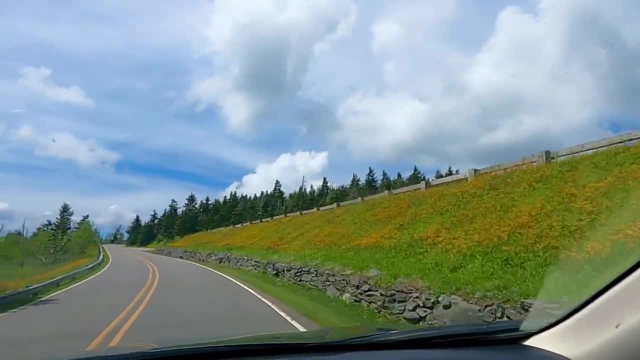 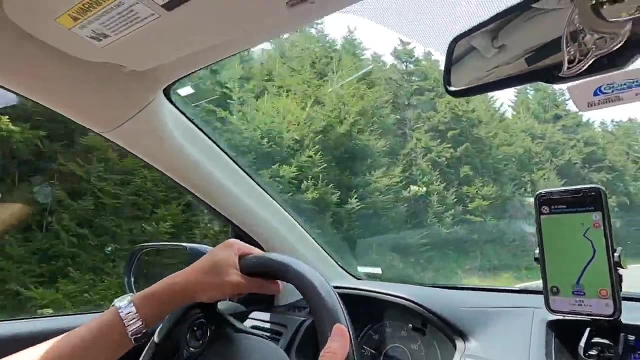 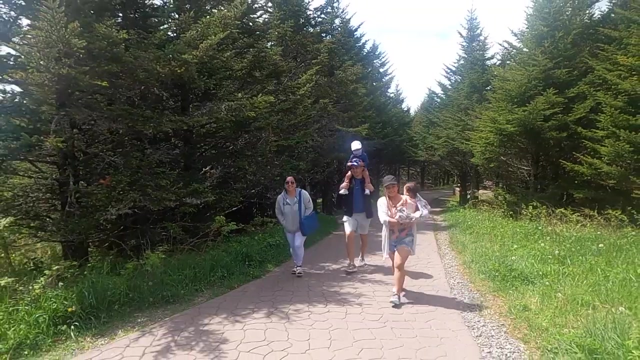 There are hiking trails, picnic spots and a Natural History Museum gift shop. NC 128 is a 4.6 mile road that ends in a parking lot close to the summit, So from the parking lot we are walking us to the summit. This is a steep 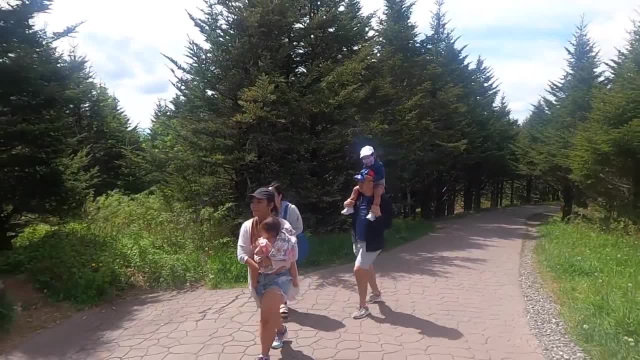 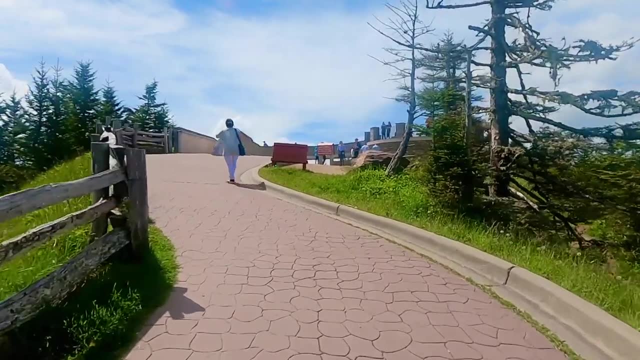 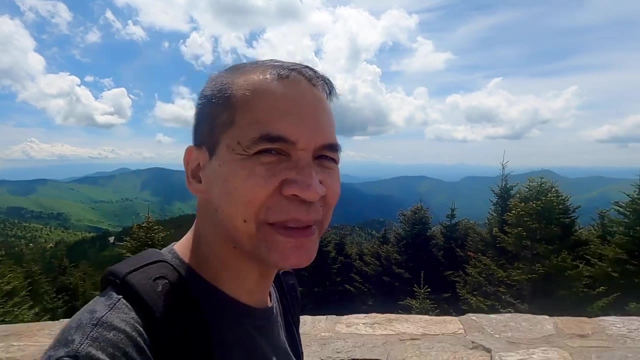 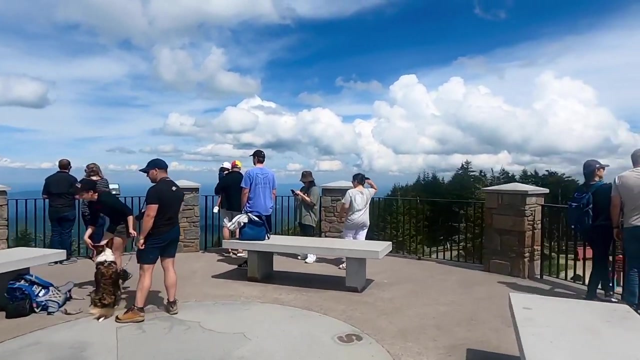 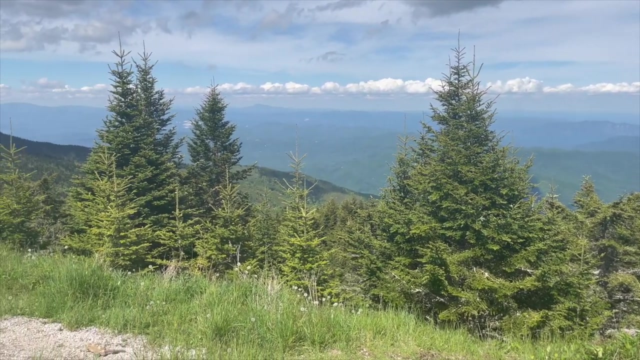 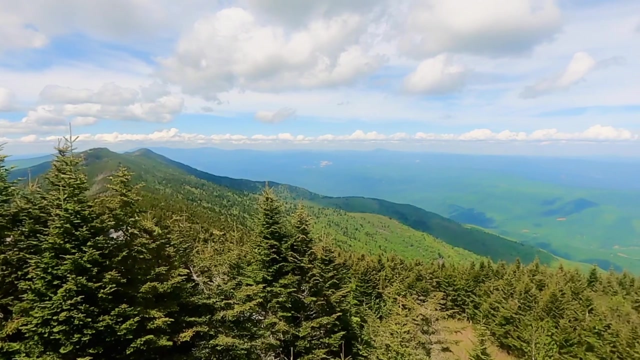 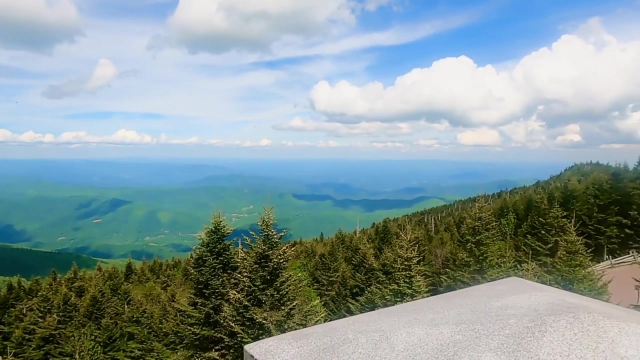 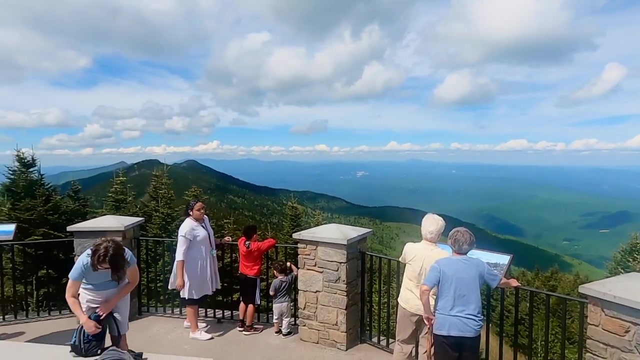 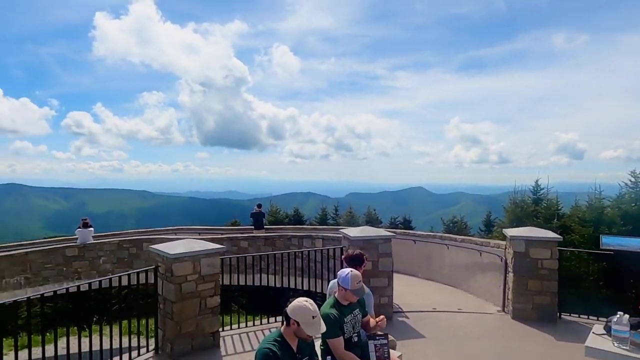 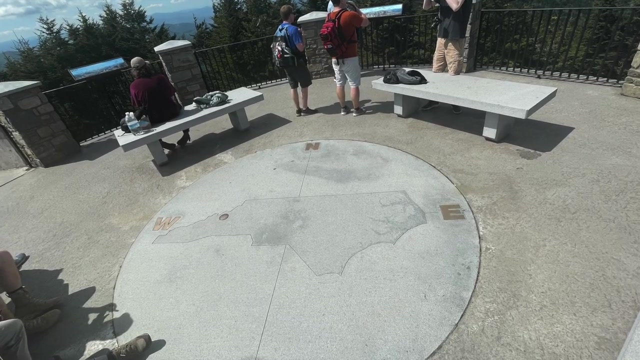 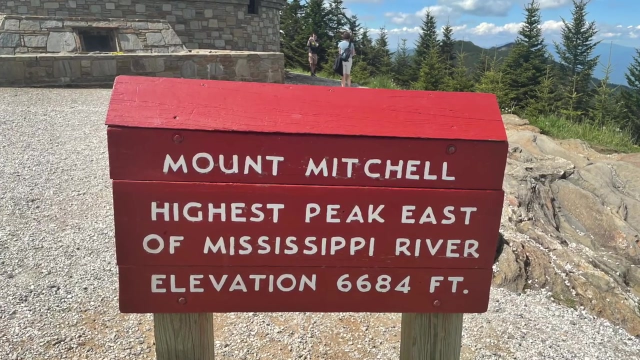 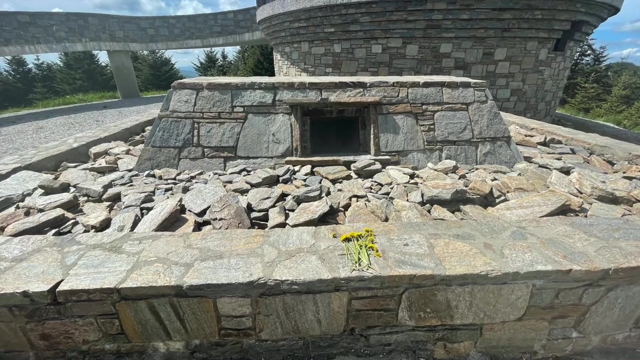 paved 980 foot trail that leads through a conifer forest to the summit. When we reached the observation deck, we were rewarded with a 360 degree breathtaking views. This is it. this is the summit and Mount Michele. you just below the observation deck, is the tomb of Elisha Mitchell, a scientist and 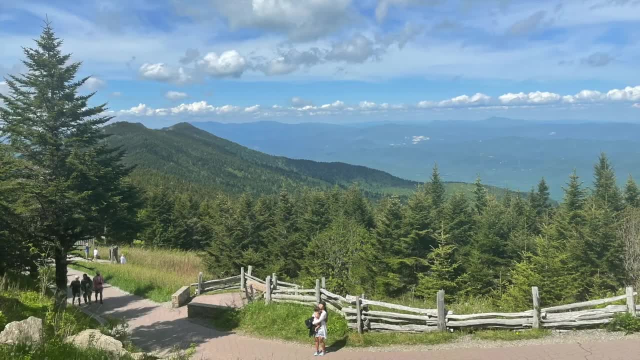 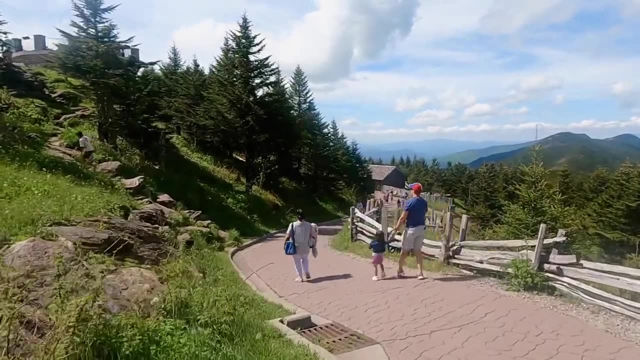 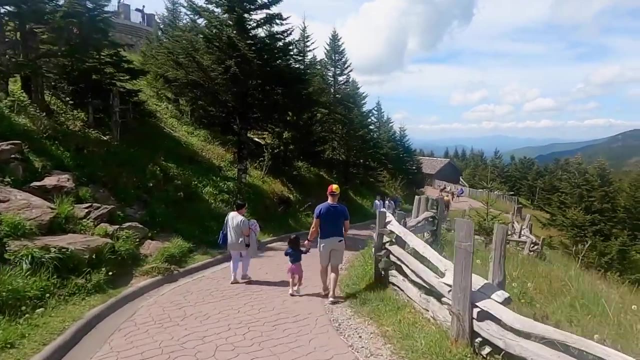 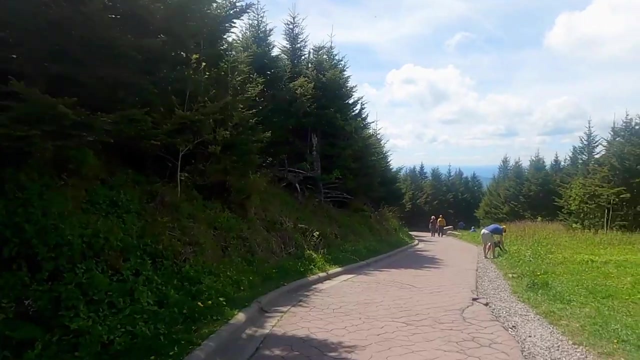 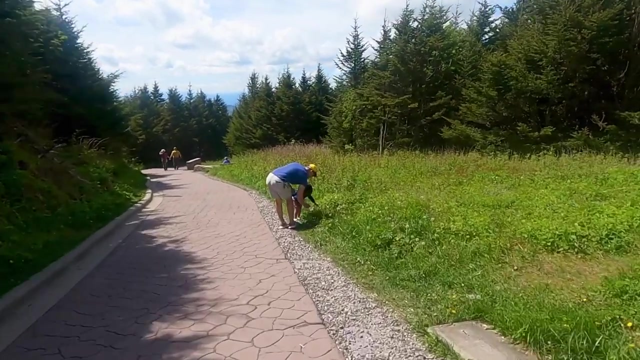 professor who died in attempt to prove that this mountain is the highest in eastern USA. This is so beautiful. here There's evergreen trees. I want to be in the picture. so beautiful. Please hit the subscribe button and the notification bell below. Thank you for watching.